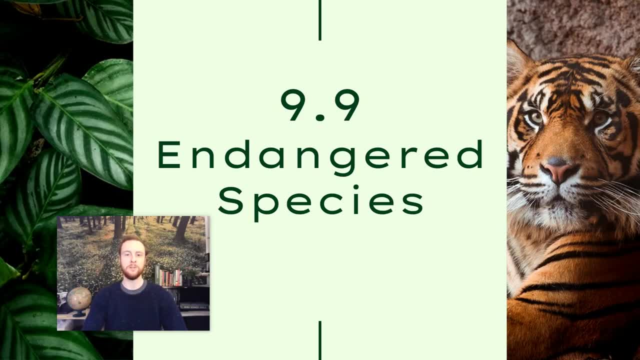 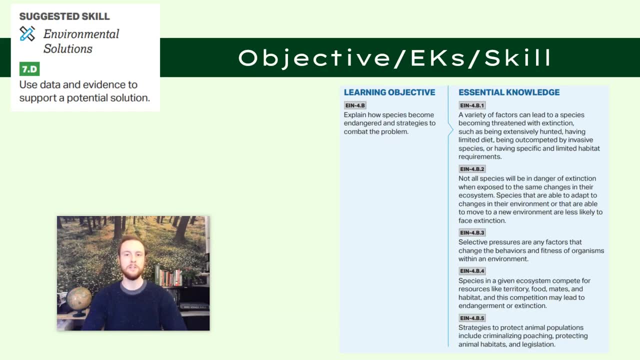 Hey everybody, it's Mr Smeeds. Welcome to Topic 9.9, where we'll be covering endangered species. Our objective for today is to be able to explain how a species becomes endangered. We can look at some of the threats to species, but we'll also look at how we can protect endangered. 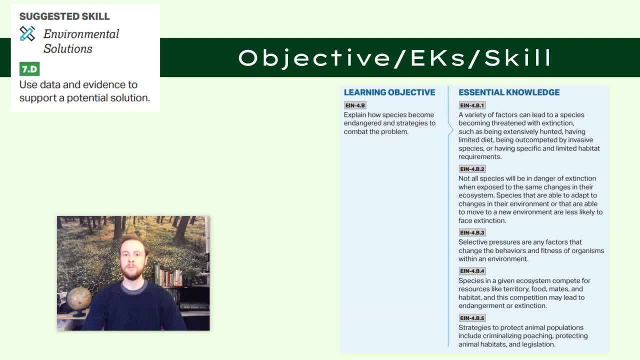 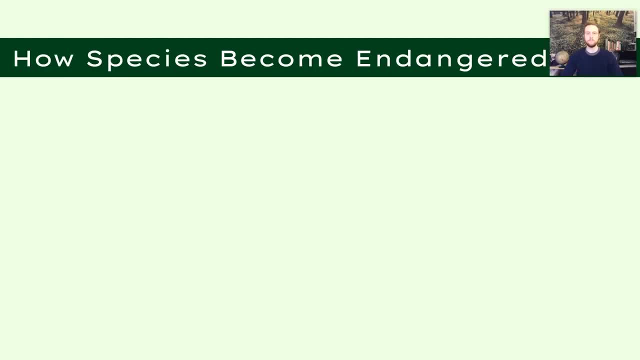 species. The skill that we'll be practicing at the end of today's video will involve using data to support a potential solution. First, we'll take a look at how species actually become endangered. One way that species can become endangered is poaching. This is the illegal hunting and trade. 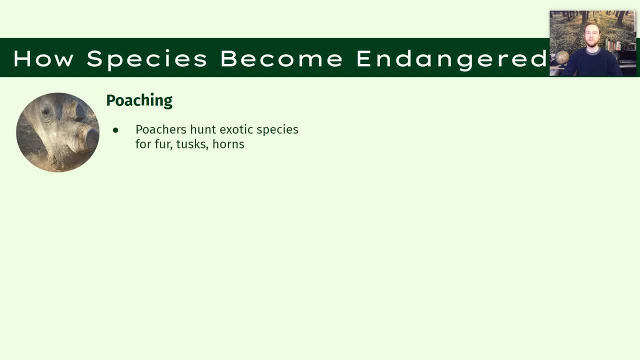 oftentimes of animals or their parts. Specifically exotic species can really be prone to poachers. This could be things like ivory from elephant tusks or the horns of rhinos. One thing that's actually done sometimes to combat this issue is to cut these valuable parts off the animals. 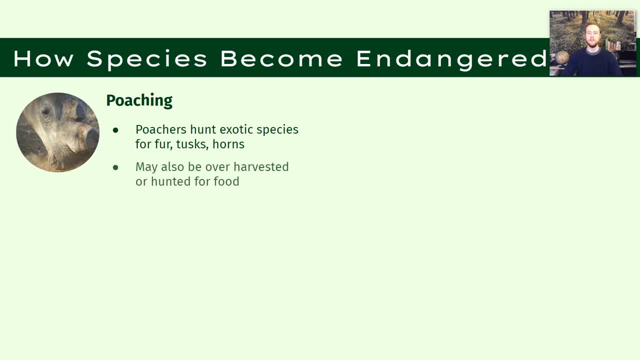 to prevent them from being killed by poachers. They can also be harvested for food. Sometimes a species becomes endangered or extinct because it's overharvested. The American bison was almost driven to extinction. It was hunted virtually to the brink of extinction. There's a great example. 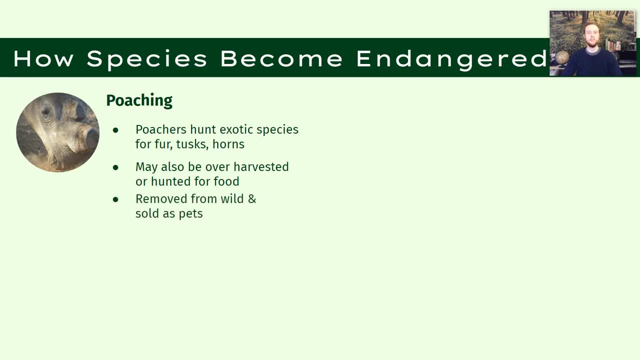 of a species that was overharvested. It can also be removed from the wild and sold as pet. There's an exotic pet trade that brings in a lot of money. Tigers are a great example of this. There's the viral show Tiger King, which obviously highlights some of the issues with the exotic pet trade. 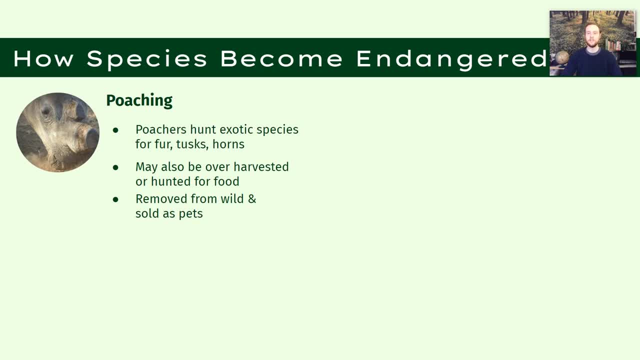 They can also be poached or taken from their natural habitat to be sold as pets. Then we have the fact that many species require very special habitats, very special resource requirements or special food needs. The quoll is a great example. If you're a niche specialist, you have. 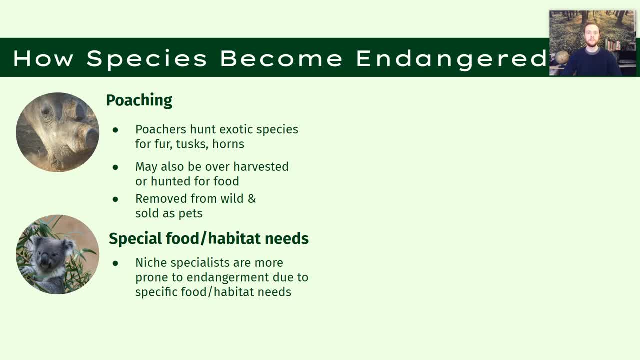 very narrow food habitat requirements. It's going to be challenging for you to survive in changing conditions. This can make you become endangered. We saw the wildfires that raged across Australia. I've heard that koala bears are considered extinct in the wild or virtually extinct. They're 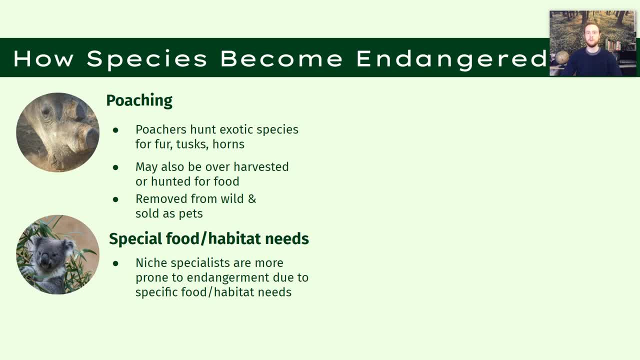 extremely threatened due to having narrow food requirements- the eucalyptus tree. That's something that can make a species become endangered or extinct. Now it's also going to make them less tolerant or less resilient. Again, we saw a great example of this when much of Australia burned. 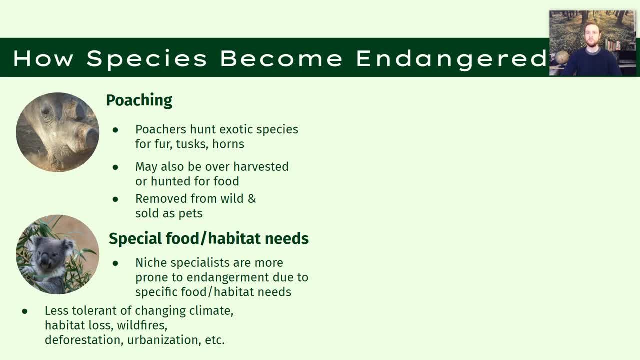 the koala bear really not being able to adapt and change to changing environmental conditions. Then we have endangered species. We've seen a lot of endangered species. We've seen a lot of invasives. Invasives pose a huge threat to native species. The zebra mussel is a great example here. 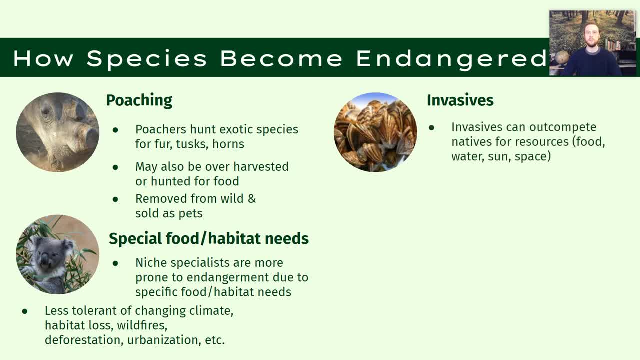 because it can out-compete native mussels. An invasive species, remember, is usually going to be very aggressive when it comes to feeding or utilizing habitats. Zebra mussels will attach themselves to basically anything. They lay up to a million eggs per female. They can reproduce. 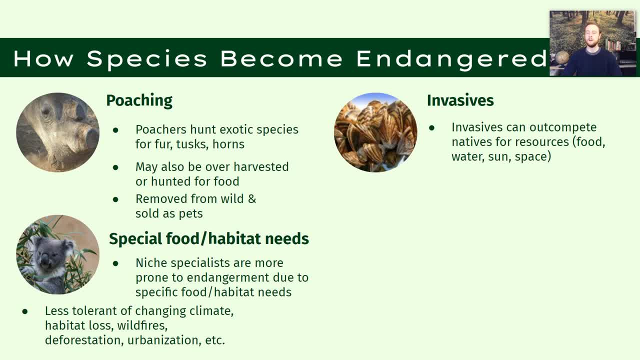 really rapidly, They can out-compete a lot of other species. Then, just again, a great example in the United States would be the zebra mussel, causing over 30 species of mussels in rivers and lakes in the United States to become endangered. One invasive can do a lot of damage when it comes. 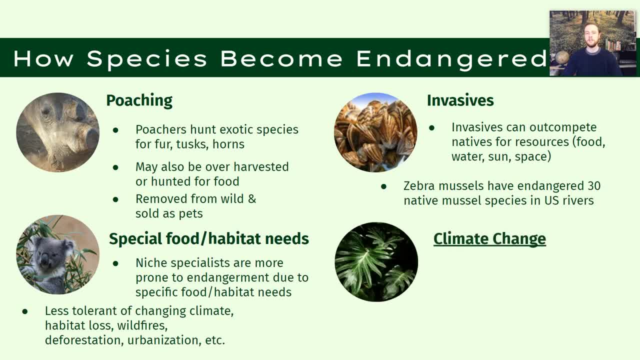 to their competitiveness. Then we have climate change. Climate change represents a huge threat to a lot of species and it's one of the drivers of a lot of species becoming endangered. When climate change occurs, it can shift the habitats of many species, Places that used to be cold enough. 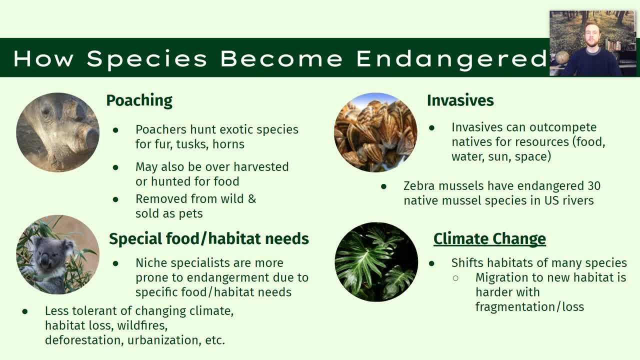 to support a thriving boreal forest may become too warm, They may start to thaw out. That could shift the habitat. Then if organisms can't adapt rapidly enough, or if the species as a whole, I should say, can't adapt rapidly enough, then they're going to be prone to endangerment or 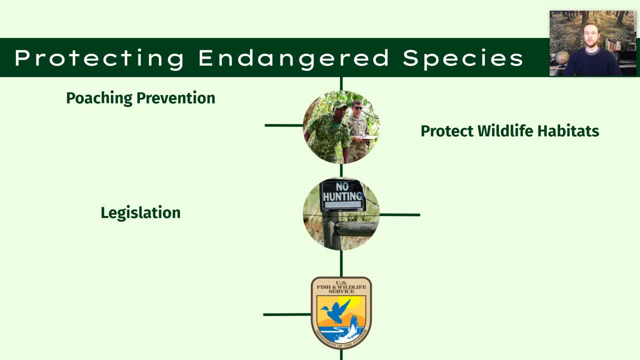 potentially even extinction. Next we'll talk about some strategies for protecting endangered species. The first thing we can do is try to prevent poaching I mentioned earlier. you can cut the valuable parts of an animal off, potentially, if that will protect it from. 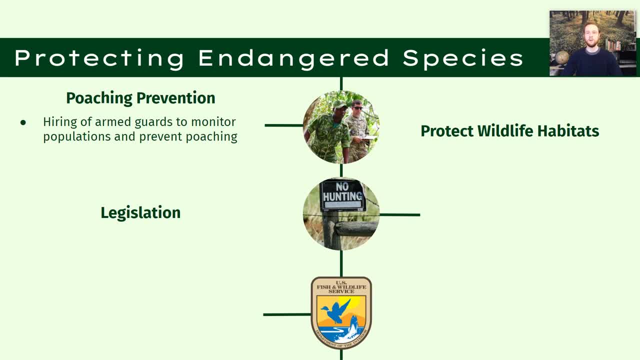 poachers, but you can also hire armed guards. We can see here armed guards and scientists working together to track vulnerable animal populations and try to prevent poaching from occurring. Oftentimes you want to arm these guards and actually give them authority to arrest or to 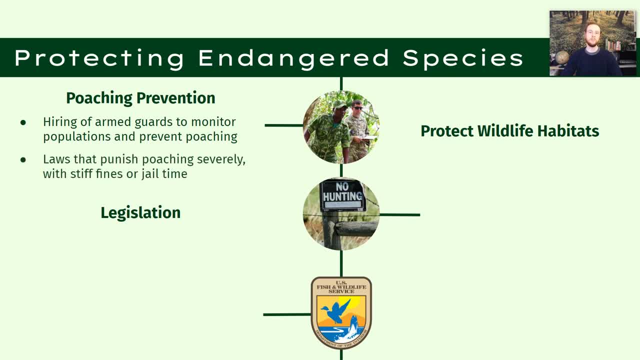 prevent illegal poaching. You can also increase the severity of penalties or fines if people are found to be poaching. You could pass laws that will put people into jail if they poach, or give them fines that are severe. You can also increase the severity of penalties or fines if people are 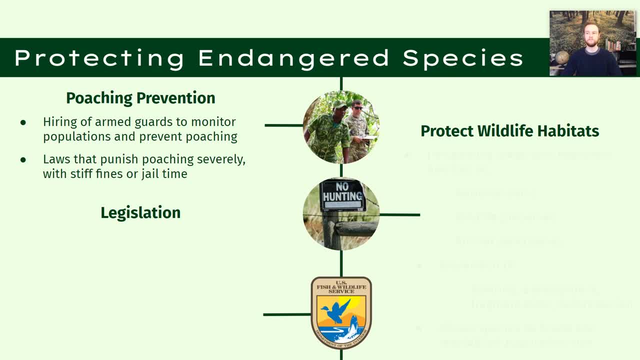 found to be poaching. You can also increase the severity of penalties or fines if people are so strict or so harsh that they will be discouraged from doing it. Another thing you can do is protect the habitat areas that wildlife need in order to survive. This is probably one of 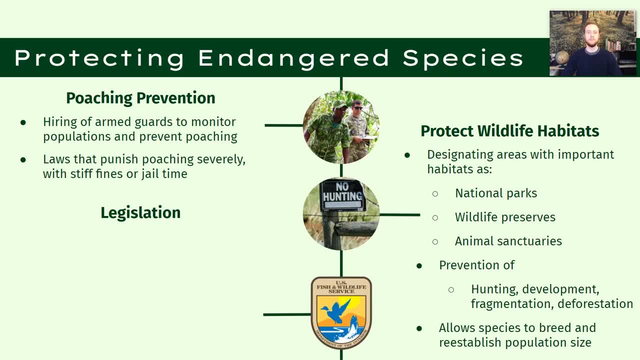 the most effective ways, because you're allowing the endangered species to have access to their natural habitat without disruption and you're enabling them time to reproduce and to repopulate on their own. This is especially important for case-selected species. Large mammals like elephants would be a great example who will really benefit from wildlife protection. So if you're 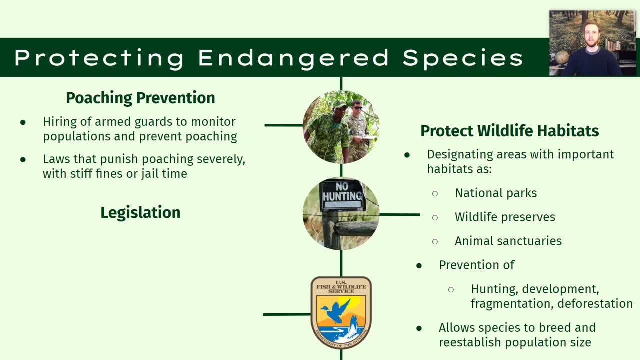 refuges, And so governments can actually purchase land. Sometimes acts or laws in their country will give them the authority to purchase land or to seize it and set it up as an endangered species habitat area, And so this could be something like a national park. It could be a wildlife preserve. 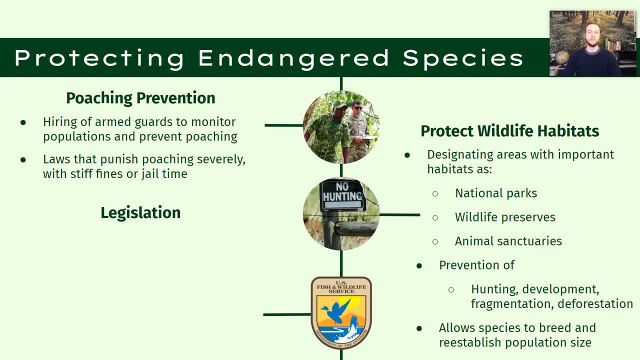 an animal sanctuary is another term we could use for this- And so this is going to help prevent, you know, illegal poaching, but it's also just going to allow that organism access to the habitat it needs, You know, animals and plant species that are endangered. oftentimes they 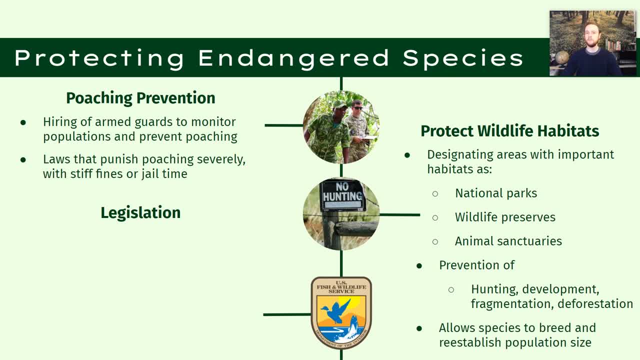 just need space and time to repopulate, And so we can give them that space and that time. And then, finally, we have legislation. So first we have sites. This is the convention on the international trade of exotic species. This is a required piece of legislation for AP environmental. 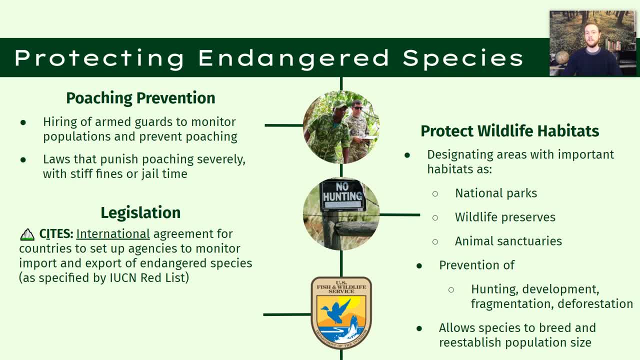 science. So we have to know this. Basically it's an international agreement, So involved you know, numerous countries all over the world basically all agreeing that each individual member country would establish its own agency within its country to monitor the import and 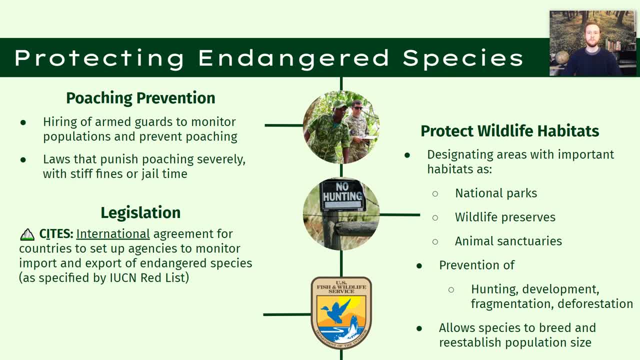 the export of exotic species. Now, this could involve their tusks, their fur and even live organisms, And so it's going to give the agencies within these countries the authority to seize those products, to prevent their import and to punish people that break this violation, or that. 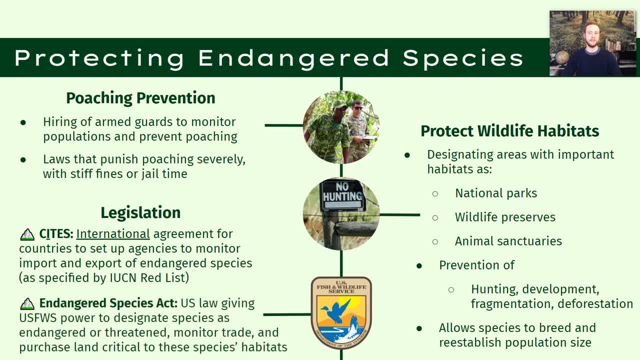 violate this law. And then we have the endangered species act. This is a piece of United States legislation, really fascinating story behind it. I don't want this video to be, you know, 20 minutes long, So I'll. I'll make another video. 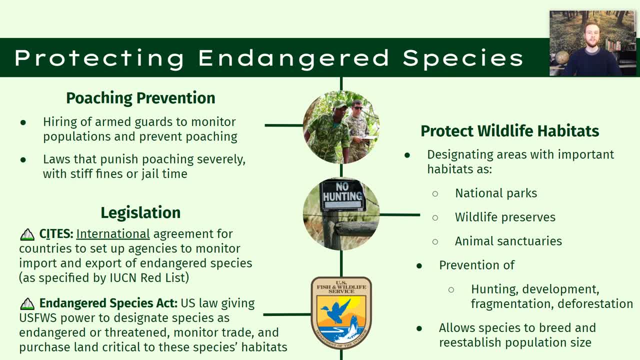 on that. but essentially we drove our national icon, the bald eagle, almost to the brink of extinction, And that was largely responsible for prompting this. but another story for another time. What we should know is that this is a U? S law that gives the fish and wildlife service. 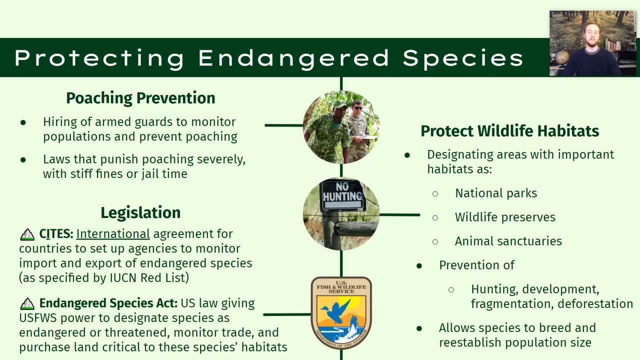 That's the United States agency responsible for enforcing it. It gives them a lot of power to basically designate species as endangered, threatened, in the United States and then to take that land and set that land up as a habitat for those species to protect them, to enable them 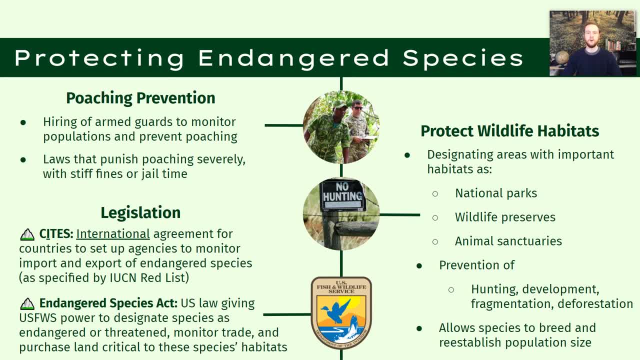 to reproduce and repopulate, And so it's a really powerful law that gives again the U S fish and wildlife service the power to actually take land and set it up and protect it, And so that is one of the most effective ways that we can try to help species that are threatened. When we refer to a 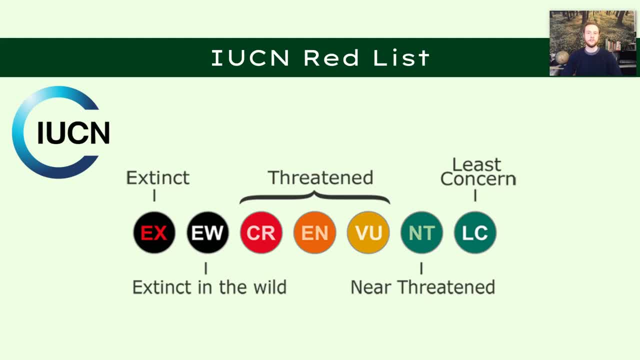 species as endangered or or as extinct. we're oftentimes referring to the IUCN red list, So it's the international union for the conservation of nature. It's the international body recognized by pretty much every major nation in terms of keeping a list of of where species are. 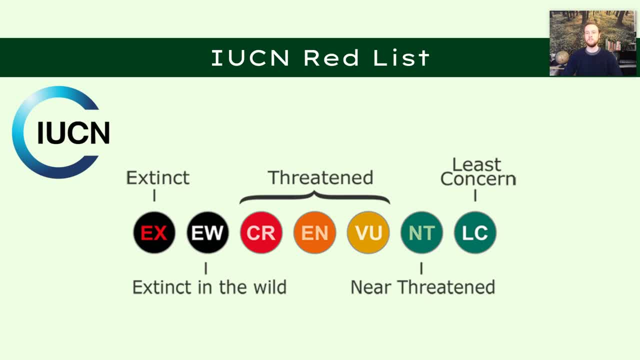 And so they assess species and then they rank them as either being of least concern. So these would be species that are basically widely abundant. They're not currently threatened, They're widely found, kind of all over the world, in their natural habitats. And then we have species. 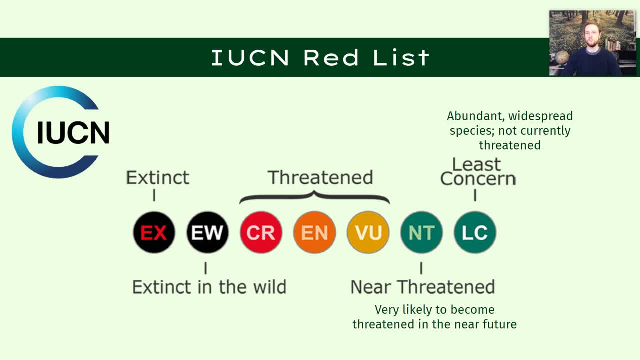 that are near threatened. These are very likely to become endangered Or threatened in the near future. And then we have a few different classifications of threatened that basically go from least vulnerable to most vulnerable or critically threatened. But these are species that have high risk of extinction in the near future. And then we do have two categories. 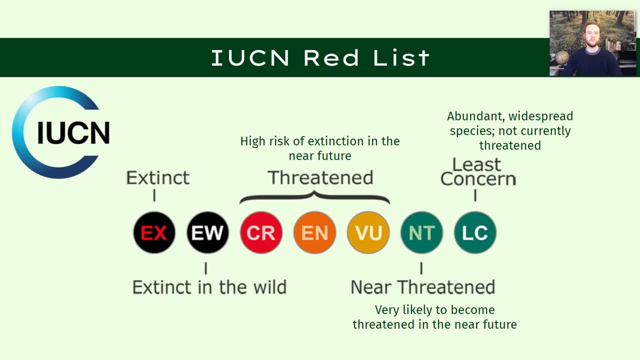 of extinction. There's extinction in the wild, where there aren't really natural populations existing anymore in their habitats. Maybe we've preserved these species in a zoo or in a sanctuary somewhere, and then there's completely extinct, So not a single member of the species left on earth. 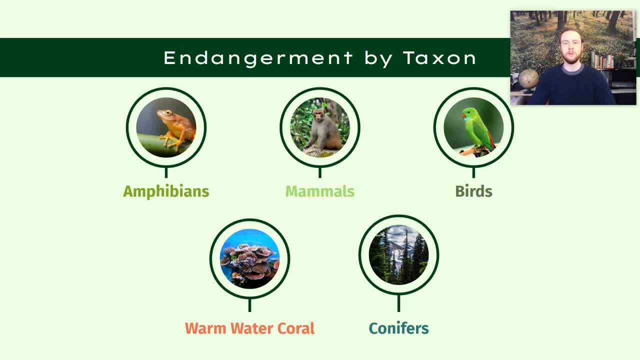 Now we'll quickly look at endangerment by taxon or the endangerment status of different groups of organisms. So amphibians are the largest group in terms of the proportion of their members that are threatened, at 41%, And so one of the reasons for this is that they're especially vulnerable to. 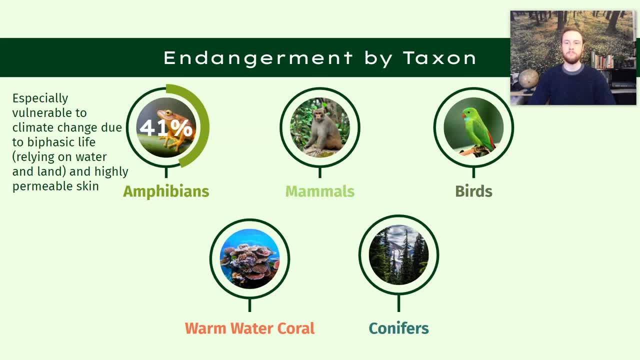 climate change and to shifting environmental conditions, because they have biphasic life. So they start out living in the water- You know, think of a frog that starts as a tadpole- and then they transitioned to living on land. They're very reliant on. 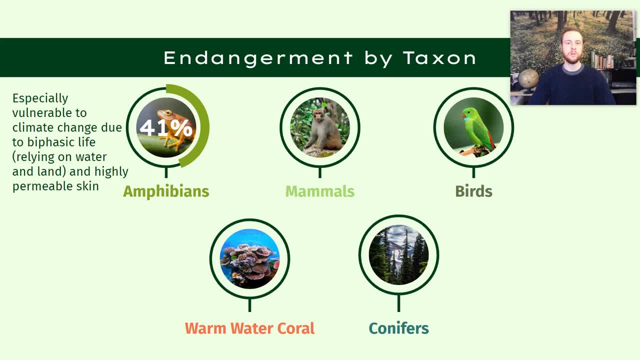 water. So, as climate change leads to some areas becoming more dry and decreasing their precipitation, there's that issue. But they also have extremely permeable skin, So they're super sensitive to pH changes in the water, to pollutants, you know, to things like acid rain. 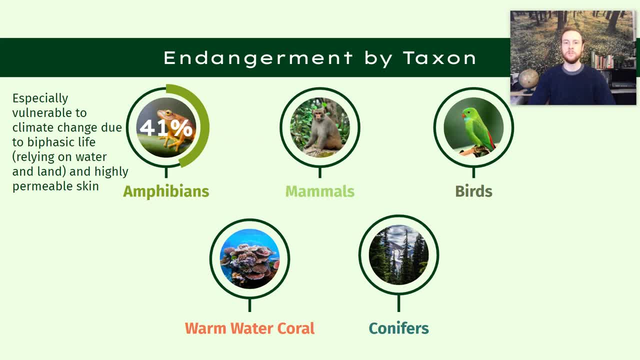 And so all of these things are going to make them more vulnerable to extinction. It's going to make more of their members threatened For mammals, about 25% of evaluated mammals are endangered. For birds, it's about 13%. For warm water coral, this is a class that has about a third of its members who have been 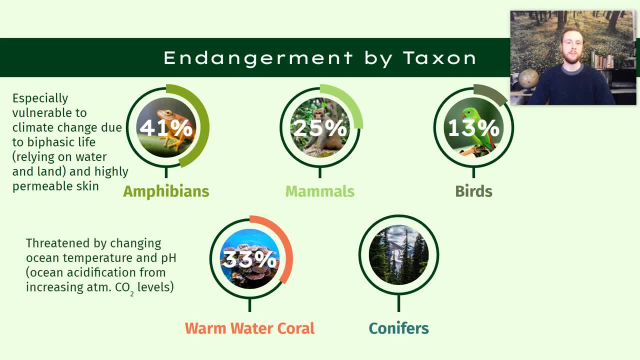 evaluated, classified as endangered, And remember that we learned about ocean acidification earlier in this unit and that's a big driver. So, as the ocean warms, one that can displace the beneficial algae that live in the coral and that supply it with sugars, But as the ocean acidifies due to 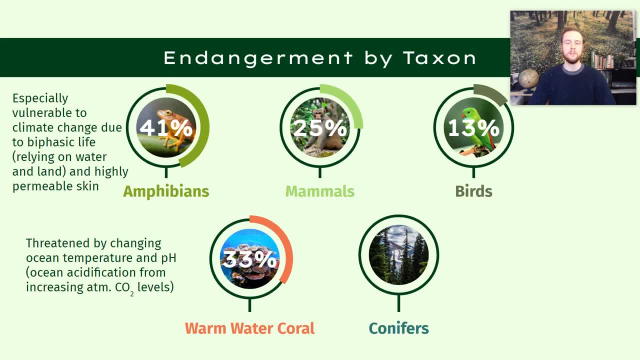 more CO2 in the atmosphere that can also drive those algae out of the coral reef. It can bleach the reef, And remember a bleached reef. it's not going to get rid of the algae, It's going to get it stressed. It's under a lot of physiological pressure and it may not recover. And then we 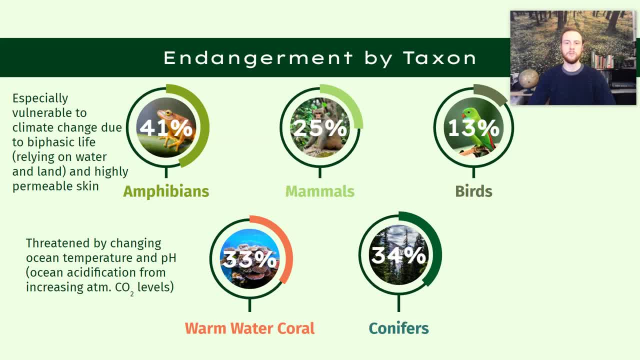 have conifers, So about 34% of all conifers evaluated are currently endangered, And this is a problem because they're threatened by disease and the expanded range of their pests or insects that, you know, damage these trees due to warming climate conditions. This is so consequential for 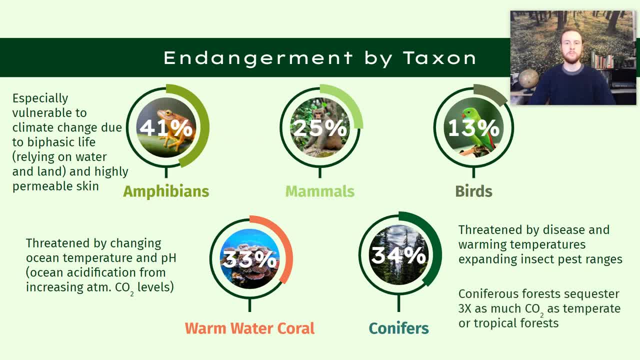 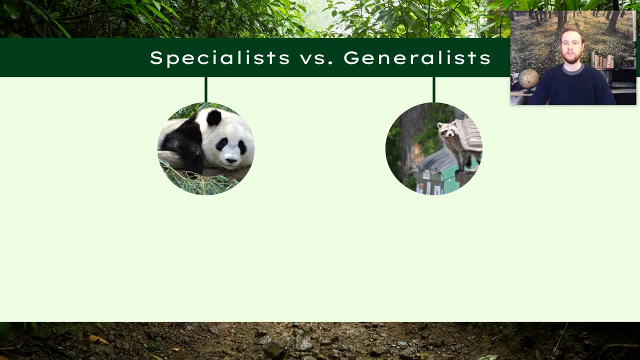 climate change, because coniferous forests sequester about three times as much carbon as temperate and forest, And so this does not bode well for mitigating climate change, because these forests are so critical to absorbing carbon dioxide from the atmosphere. We'll also take a look here at specialists versus generalists, And, as you can probably predict by now, 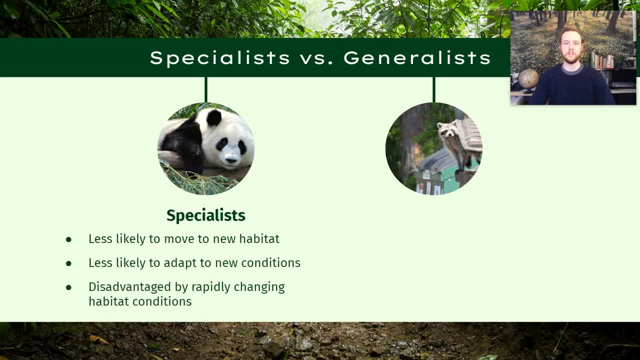 specialists are going to be a lot more vulnerable to climate change and to endangerment, And that's because they're less likely to be able to survive in a new habitat. They're less likely to adapt to new conditions or be able to utilize a new food source or new ecological niche. But if we look at 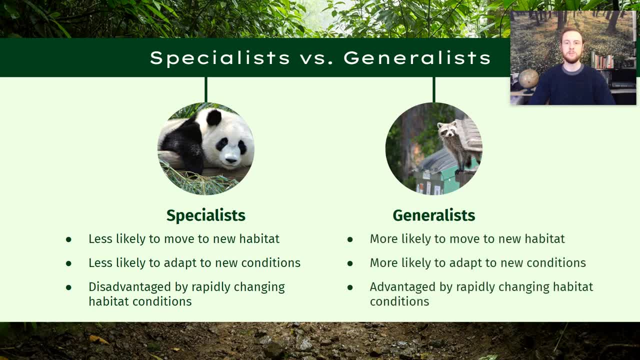 generalists, of course they're going to be, you know, advantaged in these conditions. almost. They thrive when conditions are rapidly changing because they can utilize many different food sources, many different habitat requirements, And so, as a result, specialists are going to be more. 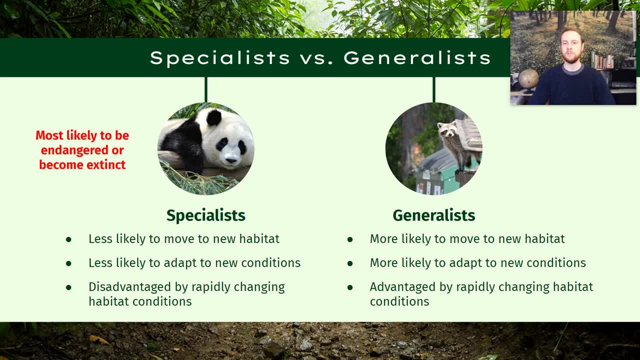 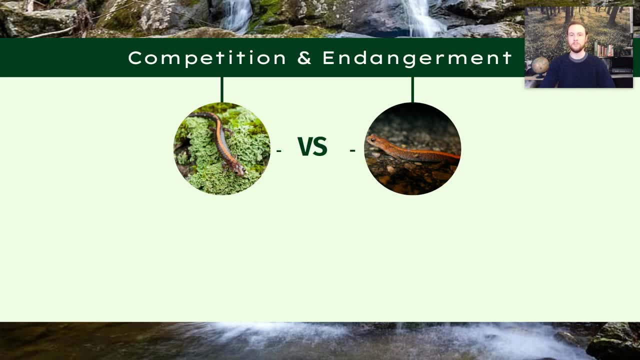 likely to be endangered, more likely to become extinct, whereas generalists are going to be far less likely to become endangered or to become extinct. And finally, we'll wrap up today by talking about how competition can actually play a factor in endangerment as well. So we have two. 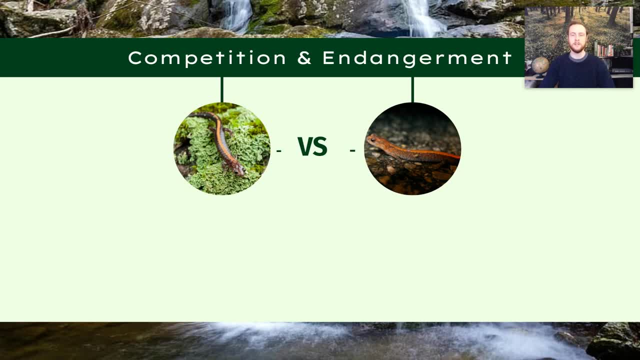 salamanders here. They may look really similar, but they are different species And competition between the two has resulted in one of them being endangered. So on the left we have the Shenandoah salamander, and this is an endangered species. Their range is currently limited to only three specific mountain peaks in 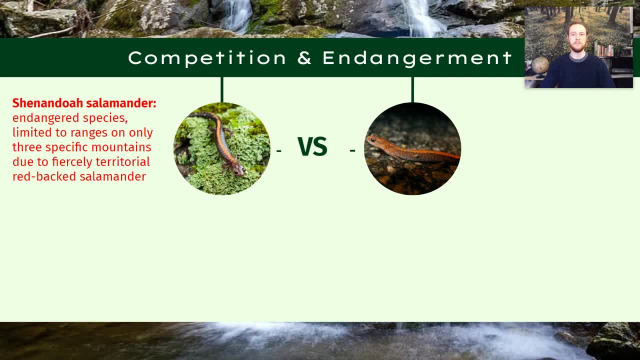 the Shenandoahs, And when they try to leave the mountain peaks to make it to lowlands, where they can expand their population, they are basically chased off by the red-backed salamander. So the red-backed salamander fiercely protects its rock. 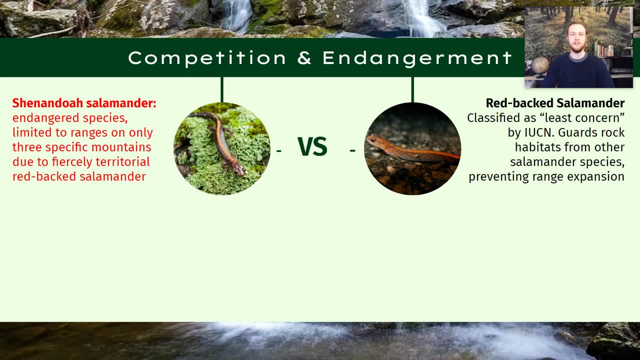 Salamanders really thrive on, you know, rock habitats that protect them from the sun and the elements and predators, And these red-backed salamanders really fiercely protect their territory, And so that's resulted in the range of the Shenandoah salamander being very limited. 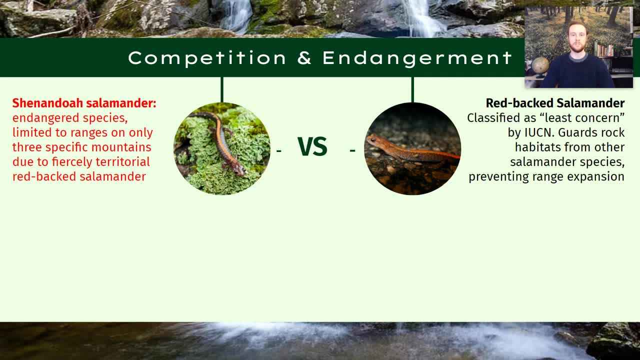 And they're basically a threatened species because of competition with the red-backed salamander. The red-backed salamander is a species of least concern. They're widely found all over the United States and in the world, in any habitat that you know fits the requirements, And so, again, competition can be a natural factor that leads. 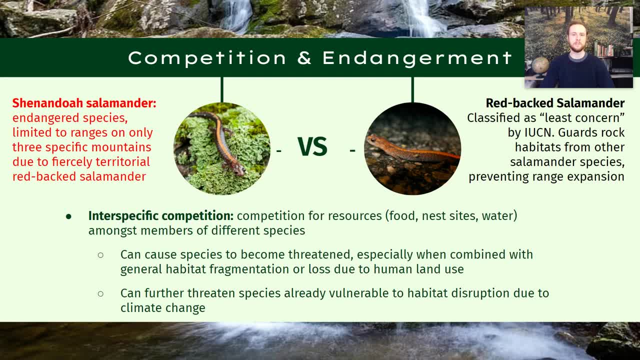 to species becoming endangered. We want to remember this, that you know, between species we call this interspecific competition. Again, this could be for food, it could be for nest sites, water, habitat. whatever it is, this can really limit the range of a species and it can cause them. 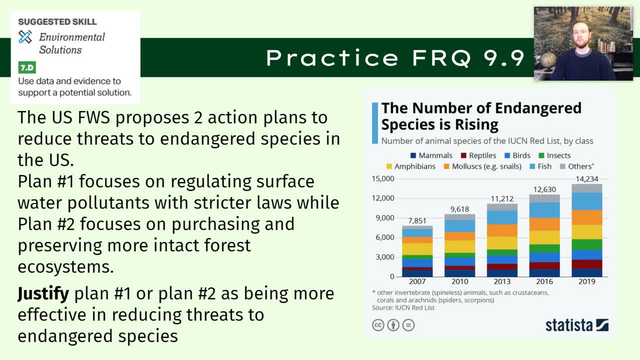 to be endangered For practice: FRQ 9.9,. I want you to take a look at this graph, which is going to show you, over time, the range of the red-backed salamander that can be endangered For practice. we want you to take a look at this graph, which is going to show you, over time, the number of members.